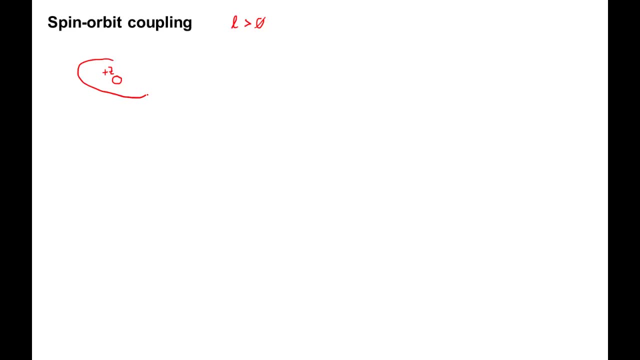 This is the nucleus with a charge of plus C. This is the orbit of the electron, and the electron orbits counterclockwise. Now let's change the reference frame. Imagine you are the electron. Then you will perceive the nucleus rotating around you. 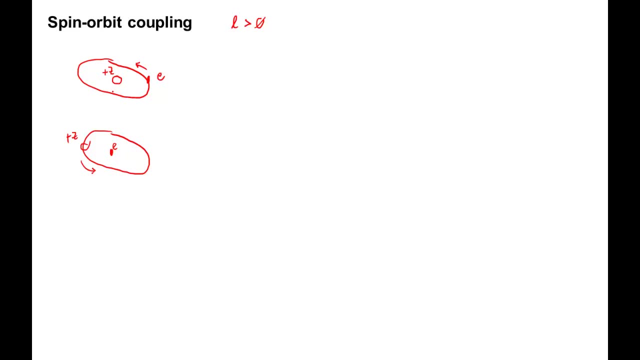 If you imagine the electron is the earth and the nucleus is the sun, you will perceive the sun rotating around the earth, even though it is the earth that rotates around the sun. Now, the nucleus is positively charged, So from the point of view of the electron, there is a positive electric current flowing. 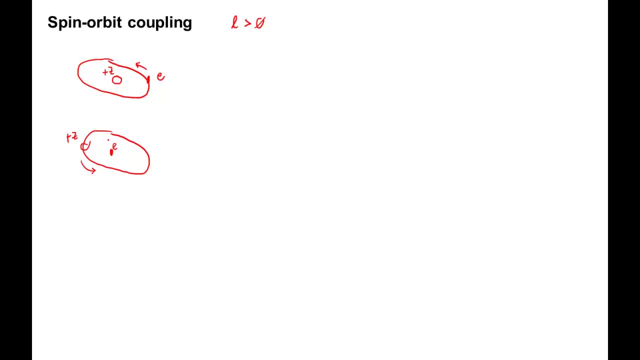 around it in a loop. Like any circular current, this current gives rise to a magnetic field. as seen from the reference frame of the electron, The field lines look like this: The magnetic field is proportional to the orbital angular momentum of the electron L. 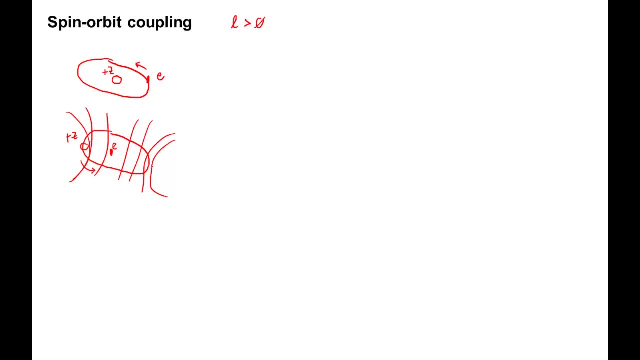 The higher L, the higher the magnetic field. In general, any particle moving in an electric field experiences a magnetic field. Thank you for watching. The electron itself is spinning and has a magnetic dipole moment. You can regard it as a tiny spinning bar magnet. 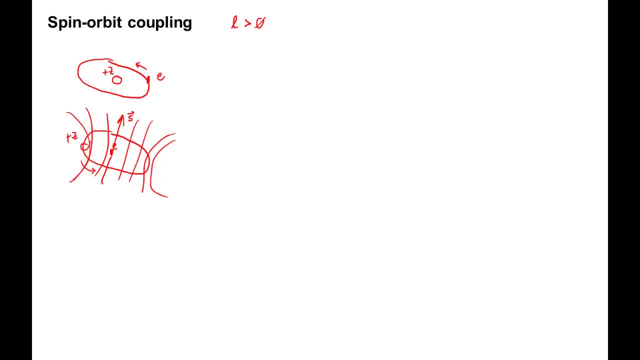 Here is the spin angular momentum vector S And here is the magnetic moment vector mu S. They are antiparallel. The electron spin magnetic moment feels the magnetic field from the nucleus. Its energy will depend on how it is oriented relative to this field. 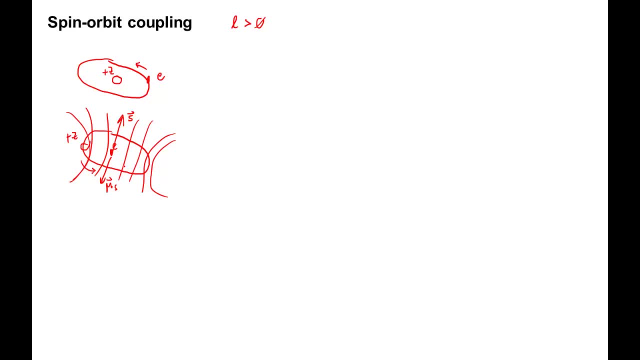 Therefore the spin and the orbital angular momentum are the same. The electron spin and the orbital angular momentum of the electron interact, although not directly, but via the presence of a charged nucleus. This is the spin-orbit coupling. To account for this coupling, we have to add an extra term to the Hamiltonian. 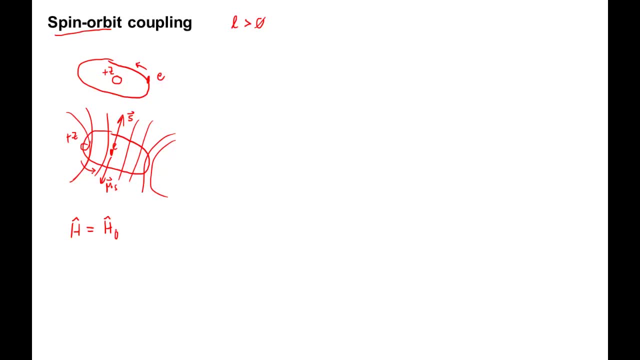 The overall Hamiltonian is H0,, which is the familiar Hamiltonian with the familiar kinetic and electrostatic energy terms, plus HSOC, the spin-orbit coupling Hamiltonian. HSOC is the spin-orbit coupling Hamiltonian. The Hamiltonian is new and is given by the interaction energy between the electric field. 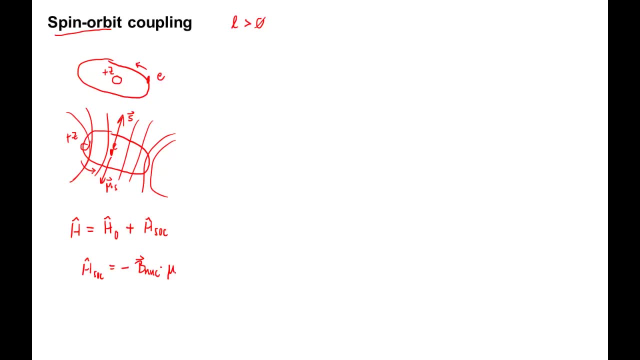 to the nucleus dot product with the spin magnetic moment of the electron. If you simplify this you'll get some coefficient xi of r times L- vector operator, dot product, S- vector operator. Basically we have a dot product between the orbital angular momentum and the spin angular. 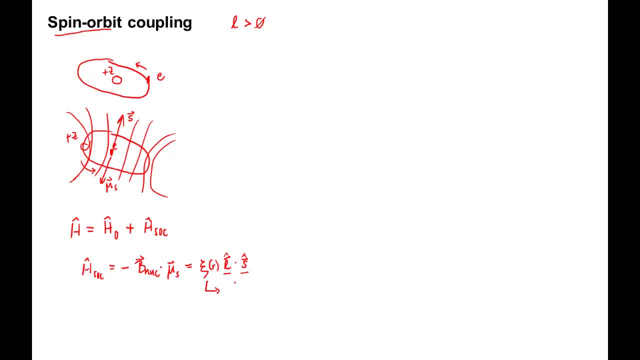 momentum. The pre-factor xi is equal to z e squared divided by eight pi, epsilon zero, m e squared, c squared times one over r cubed. If you compute the expectation value of the spin-orbit Hamiltonian for a given hydrogen wave function, you get the energy contribution due to spin-orbit coupling. 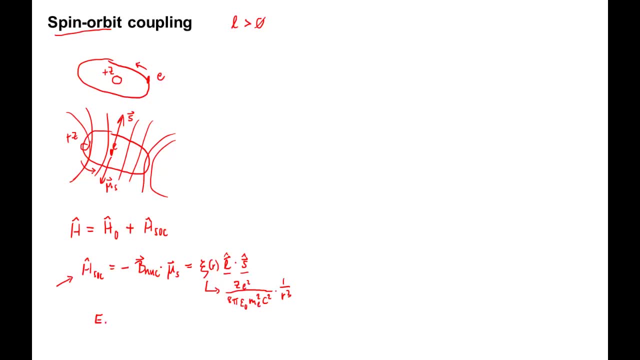 It turns out that this energy contribution, E SOC, is equal to the expectation value of the spin-orbit Hamiltonian for a given hydrogen wave function. you get the energy contribution due to spin-orbit coupling. It's proportional to z to the fourth, to the nuclear charge raised to the fourth power. 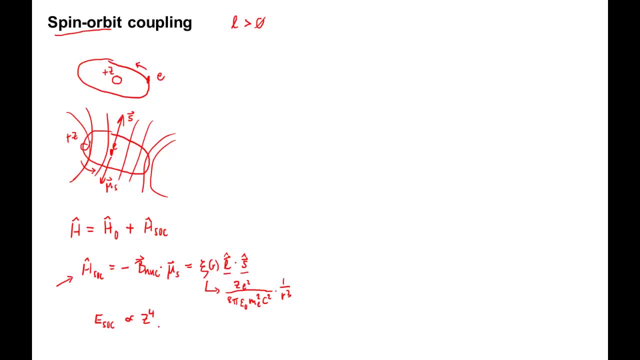 Therefore, even though the spin-orbit coupling is almost negligibly small for hydrogen, it is of dominating importance for heavy nuclei further down the periodic table. Let's illustrate the spin-orbit coupling with a simple picture. Here's the nucleus and the electron orbiting around it. 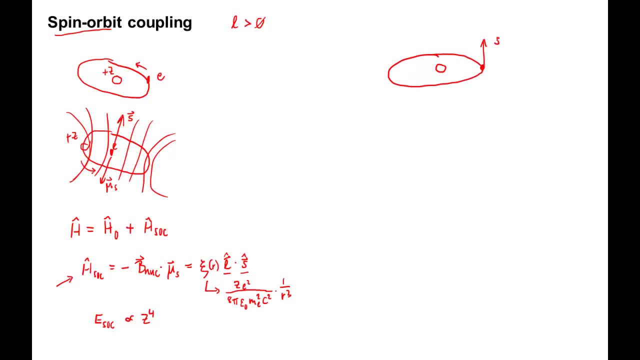 Let's have a spin-up state for the electron. So this is the spin vector And this is the spin vector And this is the spin-angular momentum vector. S It points up, If the electron rotates counterclockwise, its orbital angular momentum vector points. 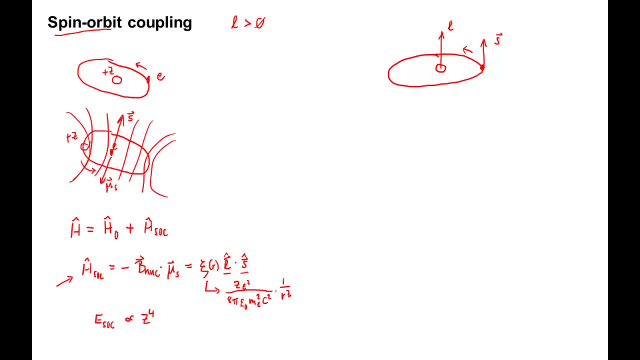 up as well. We draw it at the position of the nucleus. The two angular momenta are parallel, So the dot product in the spin-orbit Hamiltonian is positive and the energy contribution is positive as well. This relative orientation has high energy. 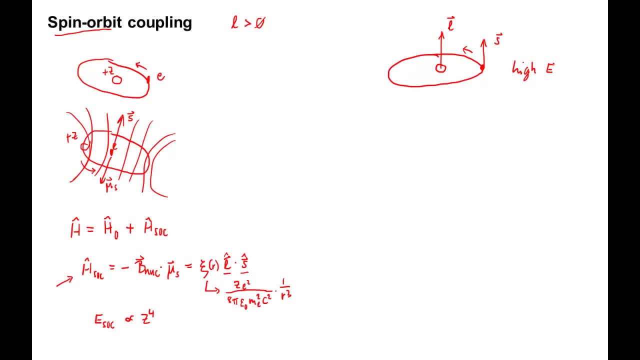 On the other hand, let's look at the spin-orbit Hamiltonian. Let's have a spin-orbit coupling. On the other hand, let's look at the spin down state in the same orbital situation. The dot product in the spin-orbit Hamiltonian is negative and we have a negative energy.